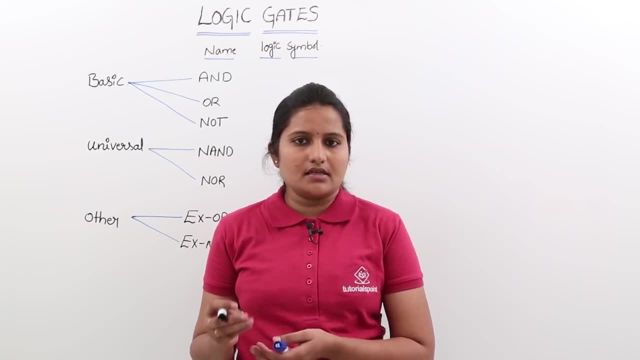 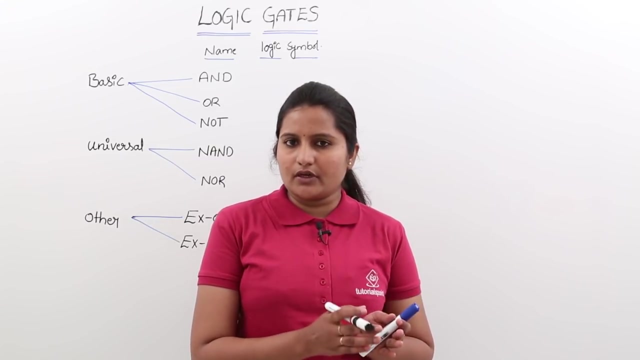 In the same way to allow or deny these digital signals, logic signals. these logic gates are used, For example, if you are using any gate, So that gate particularly allows specific combination of input signals. Generally, these logic gates are used to define a Boolean expression. this, whatever. 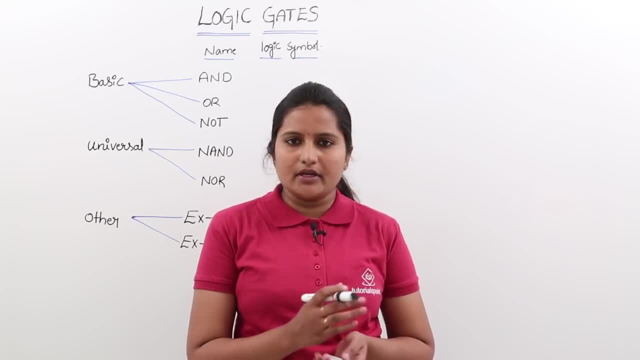 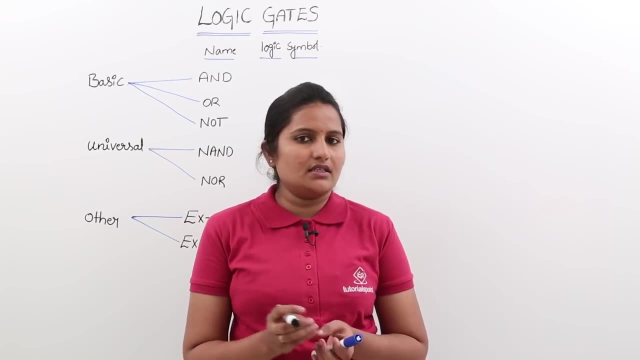 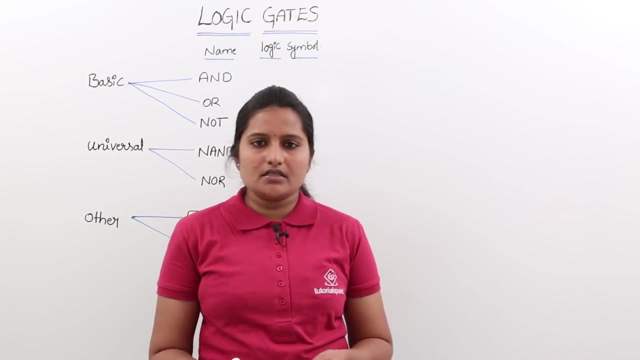 output of logic gate is there. that is a Boolean expression. So these are the basic building blocks of any digital circuit. simply, we can say: these are the main building blocks for any digital circuit. If you want to design any digital circuits, without logic gates we cannot design any digital circuit. 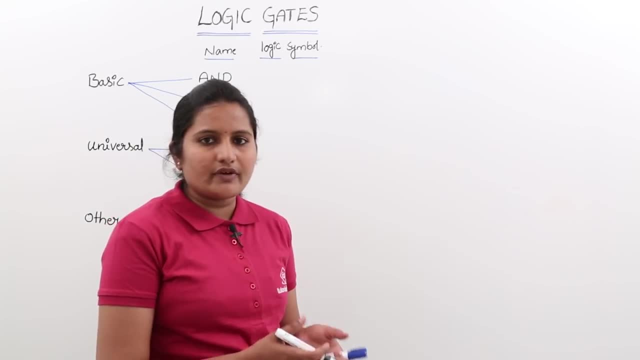 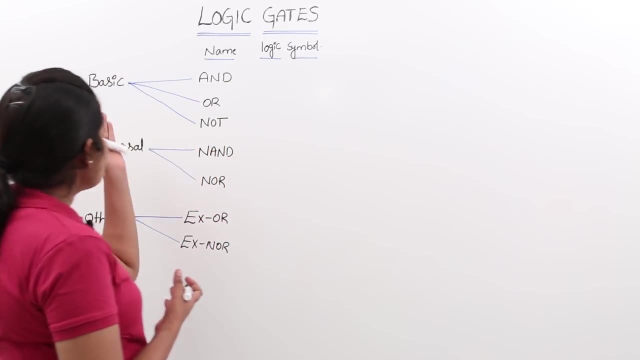 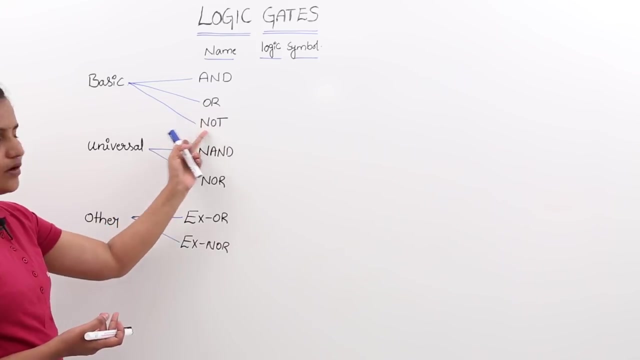 So now we will skip into. how many types of gates are there, what are the logic gates, basic logic gates, and is there any other gates? are there? let us see here. So see, here we are having basic gates as three basic gates. those are AND gate, R gate and NOT gate, And we are having two universal gates. those two universal gates are NAND gate and NOR gate and we are having two other gates like XOR and XNOR. So now these are the names of logic gates. So here why we are calling these two NAND and NOR gates as universal gates means by using these two NAND and NOR, we can realize 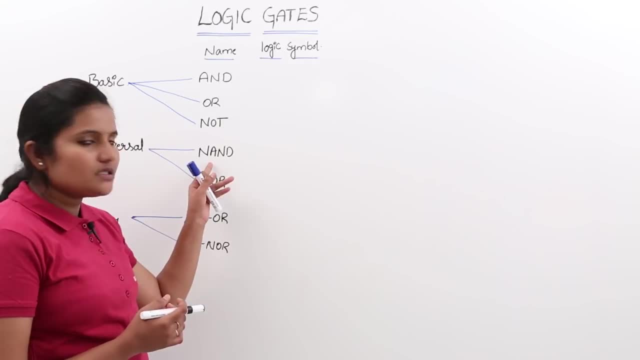 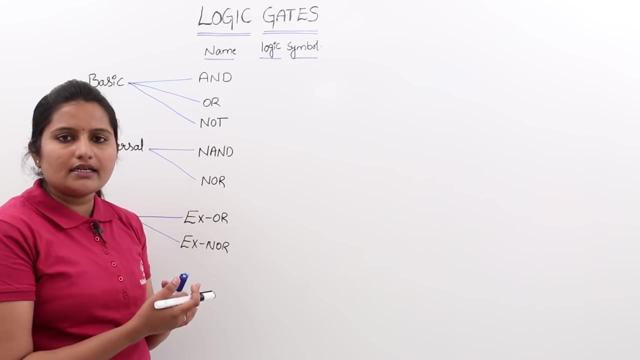 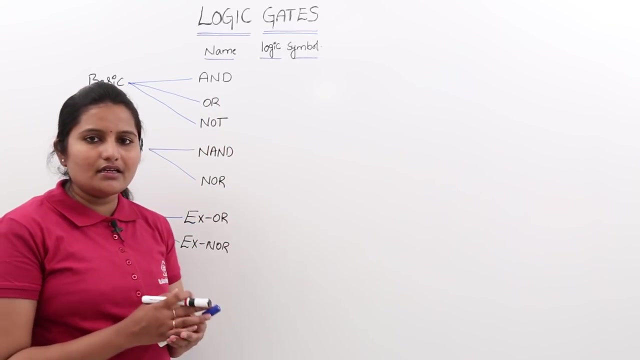 all other gates. For example, you can realize AND gate by using NAND gates combination. you need a couple or more NAND gates to realize AND gate. So, like that, you can realize R, NOT and XOR and XNOR by using NAND gate realizations. So, similarly, by using NOR gates. 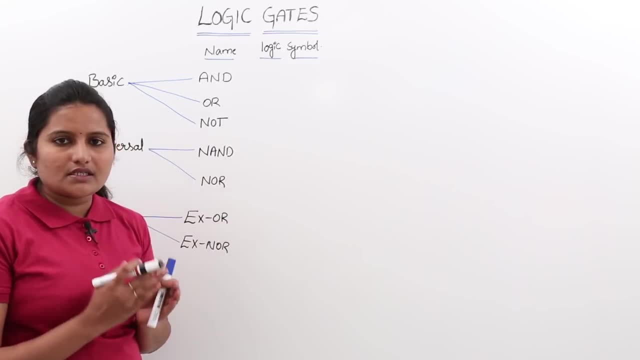 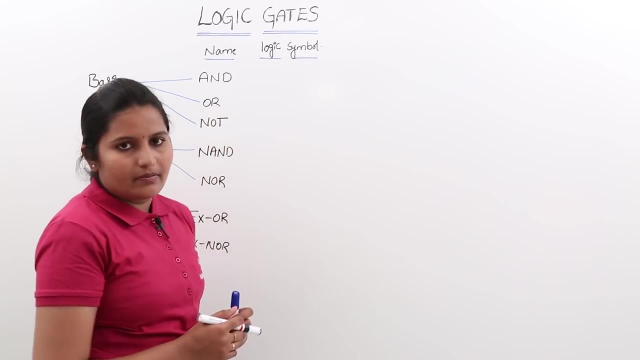 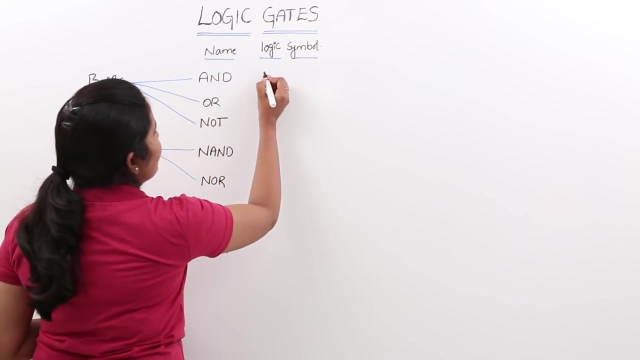 you can realize all other gates. So that is why we are calling these two gates as universal gates. Now we will see logic symbols. So let me draw logic symbols for each and every gate here. So for AND gate, the logic symbol will be like this: So this is the logic symbol. 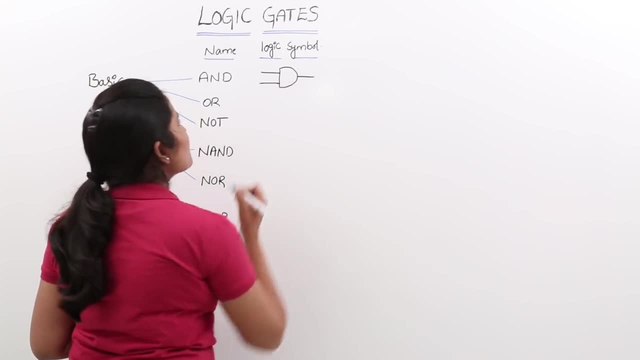 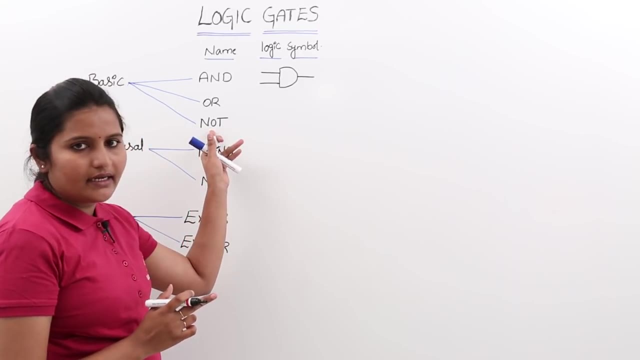 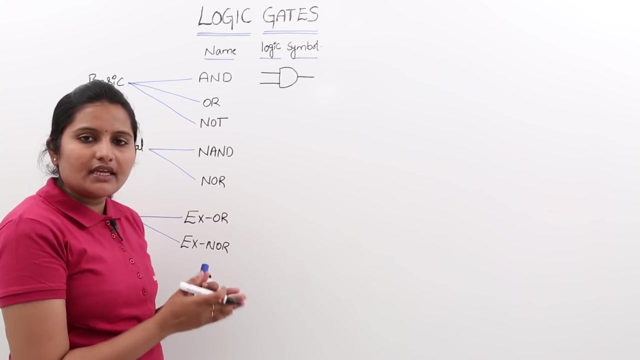 for AND gate. So it is having more than 2 inputs. it may have more than 2 inputs and only 1 output. Except this, NOT gate, all other gates can have n number of inputs or excitations. We can say inputs as excitations and output as response. So all gates can have n number. 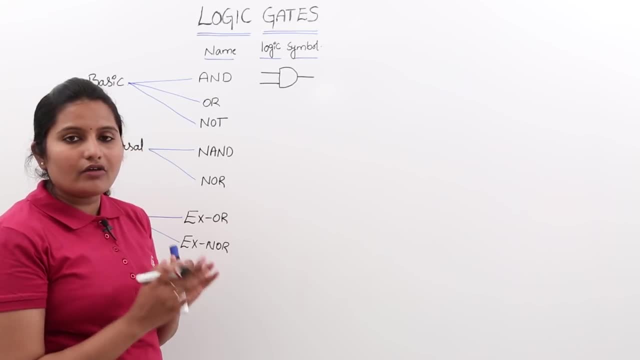 of excitations and only 1 response. Always for any logic gate, the response will be 1.. So that means only 1 in number. the response is 1 in number. So here the logic symbol will be like this. So this is the logic symbol for AND gate. 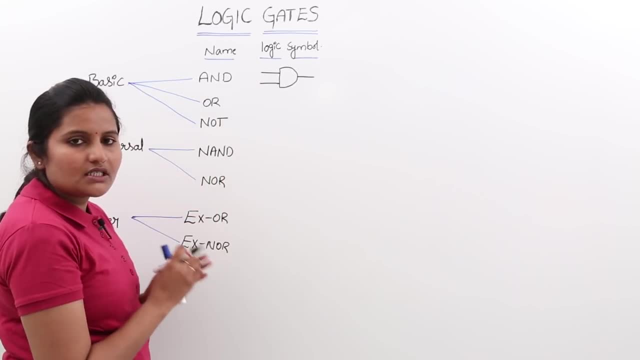 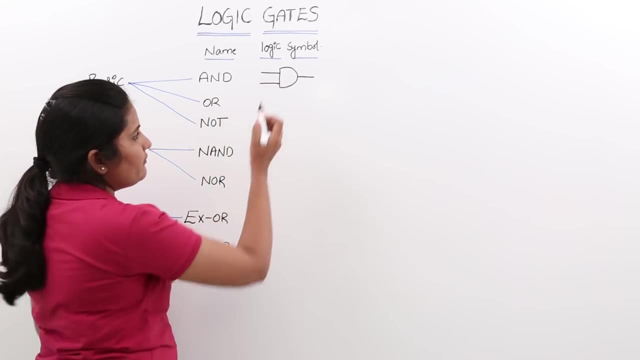 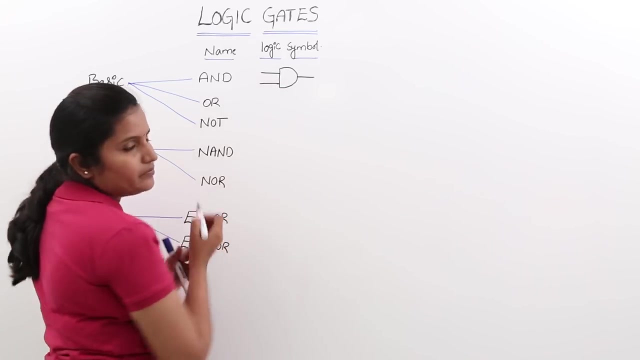 For example I am taking 2 input gates logic symbol for 2 input gates you may have n inputs, Just varies the input lines. For example, if it is symbol for 2 input AND gate, the 3 input AND gate may have 3 lines here And n input AND gate may have n input lines at. 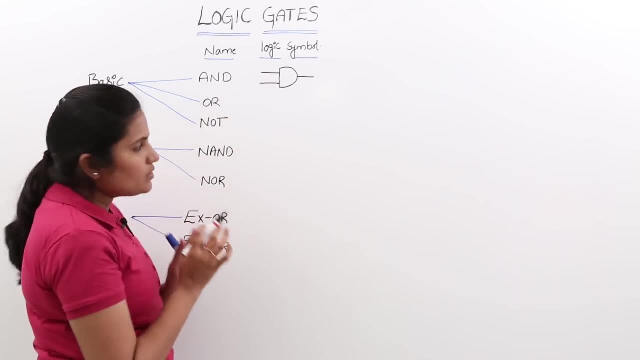 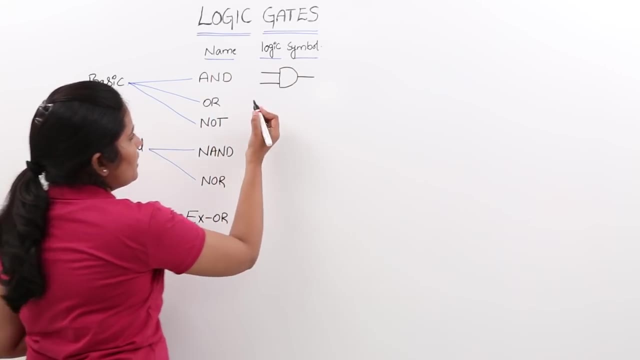 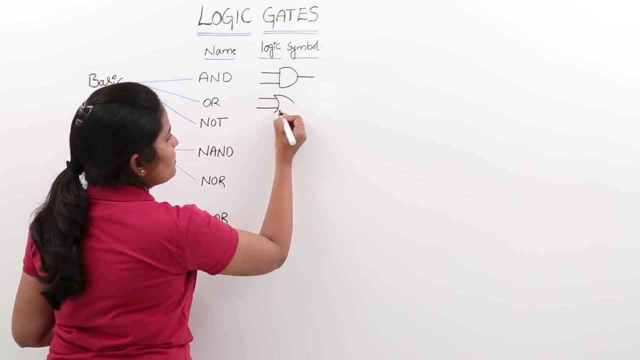 the input end. Here you may have n inputs. So here this is logic symbol for AND gate. Now we are going for logic symbol for R gate. So for R gate the logic symbol may be like this: So this is the logic symbol for R gate. So here these 2 are inputs. So 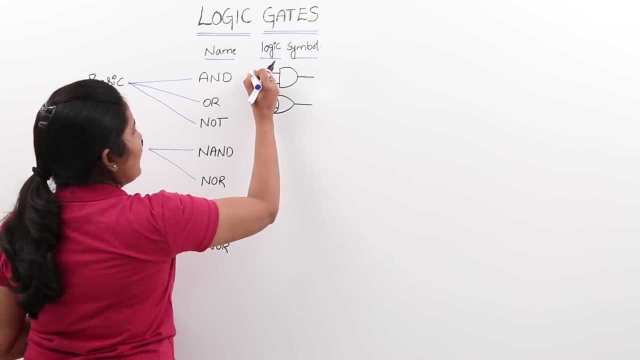 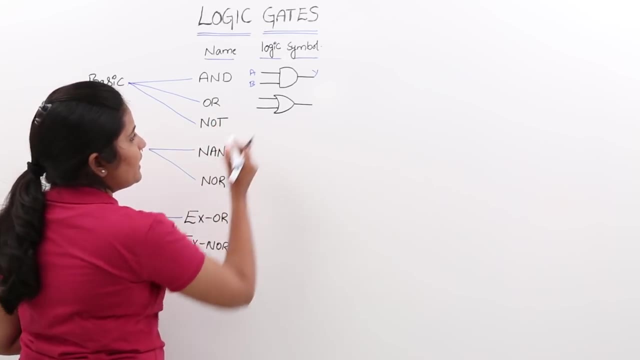 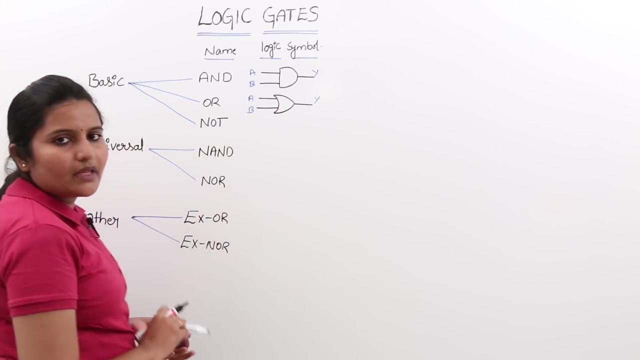 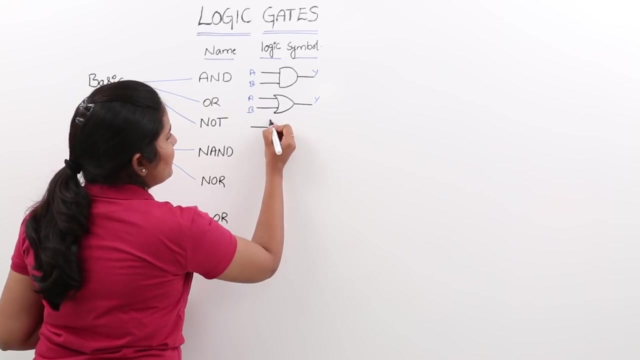 you can say: these 2 inputs, like A and B, this is output. Y. Similarly for this R gate, these are the inputs and this is output. So similarly we are having logic symbol for NOT gate. So I already told you, for NOT gate there is only 1 input and 1 output. This output may. 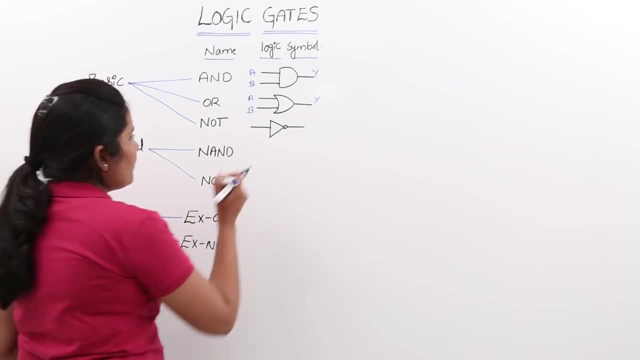 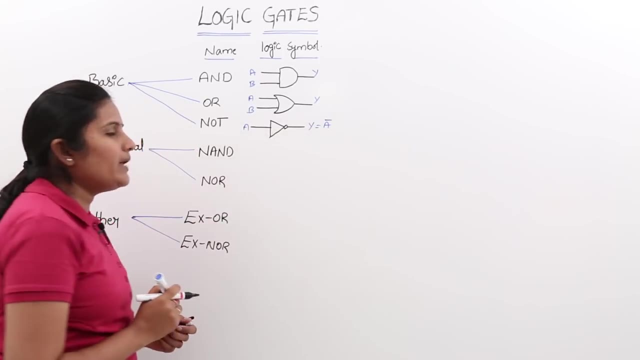 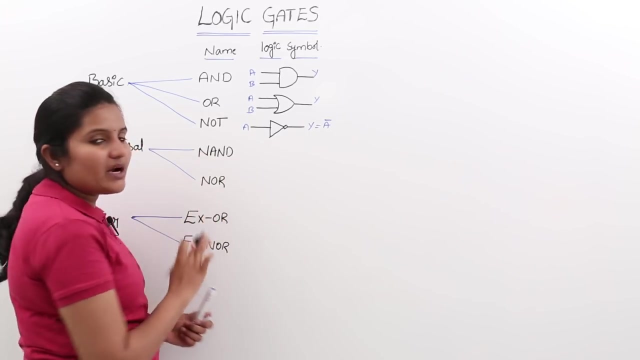 be the complement of input. For example, if you are providing A here, your output Y is equivalent to A bar. That means complement of input. we given. So see here for NAND gate. NAND is nothing but NOT end, So complement of end is nothing. 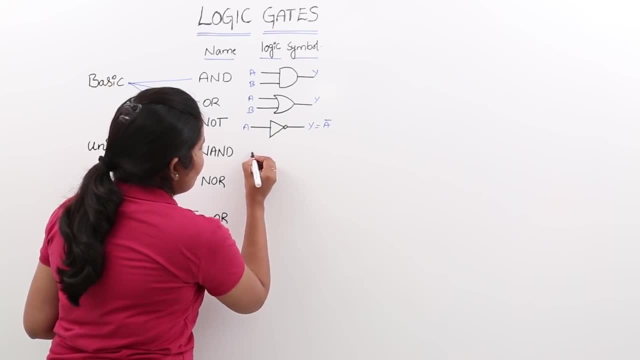 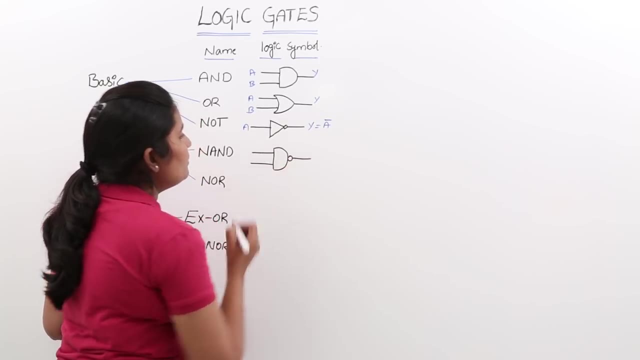 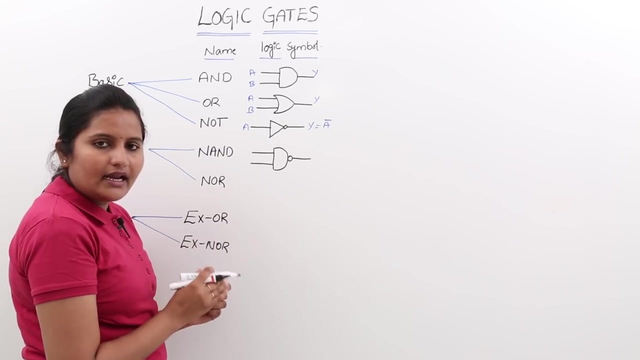 but NAND. So here we are going with the same symbol as END gate, with some NOT. So this will provide you NAND gate. So this is somewhat similar to END gate. So, as I told you, NAND gate is equivalent to END plus NOT. You are taking N and NOT gate. This is the equivalent. 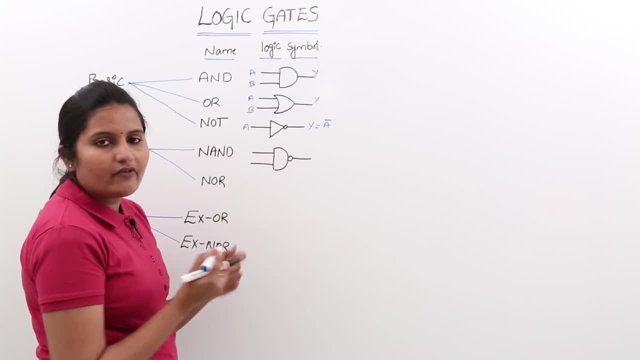 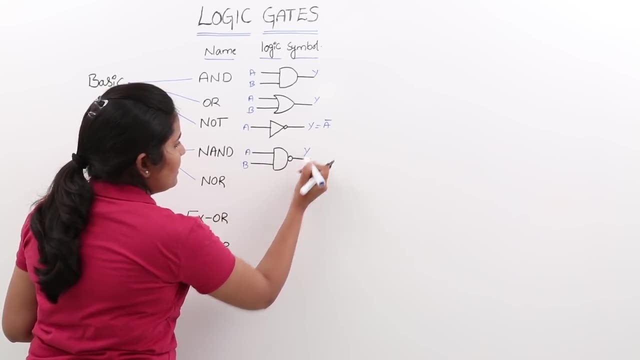 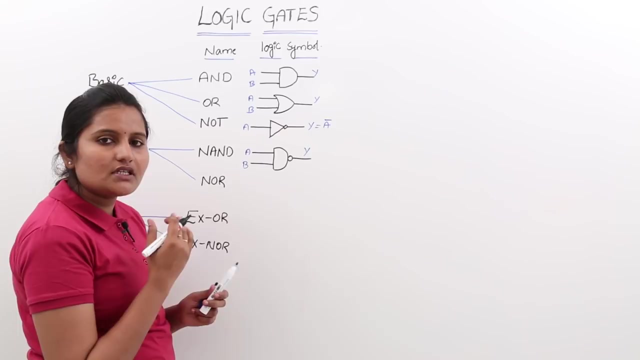 of END plus NOT gate here. So this will provide you logic symbol for NAND gate. So see, here these are the two inputs, A and B, and here output is Y. here So now for NOT NOR gate. the logic symbol is somewhat similar. 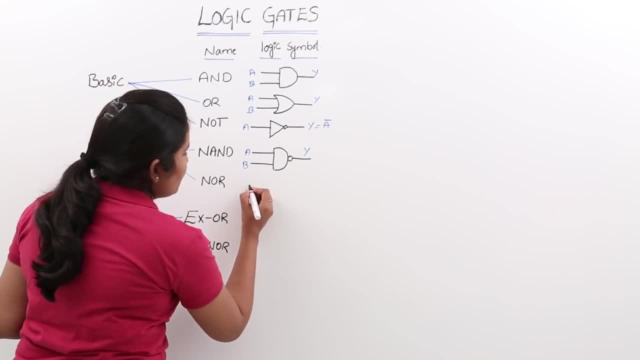 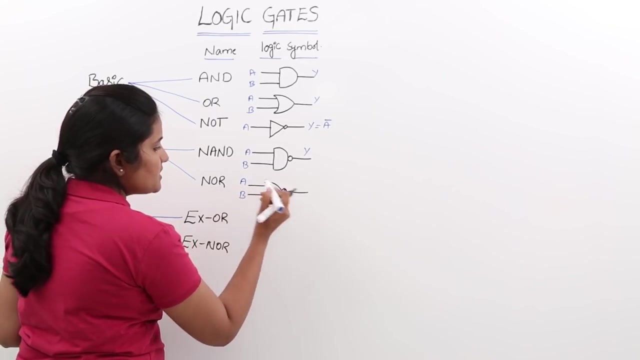 to R gate with NOT. So here the logic symbol for NOR gate will be like this. This is somewhat similar to R gate with NOT. This is symbol for NOR gate. Here also we may have two inputs. So as this is two input, NOR gate, we may have two inputs and one output. You can observe here: 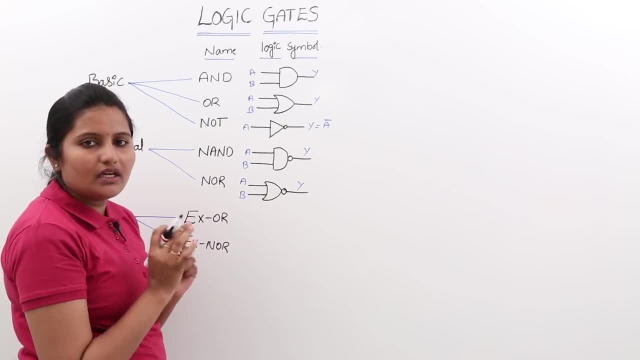 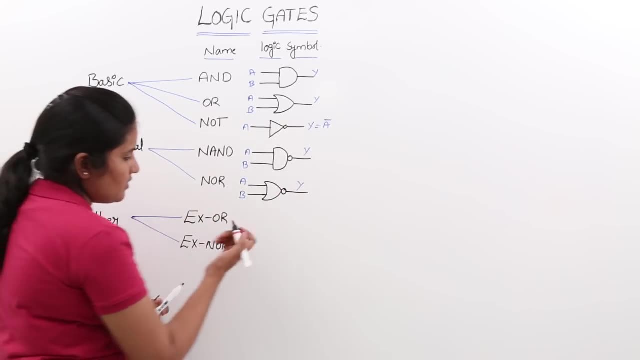 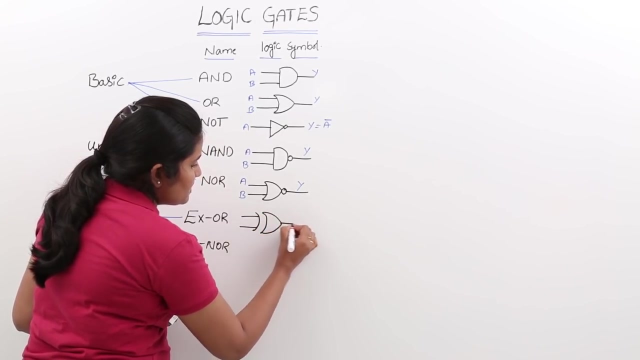 for each and every gate, the output is only one. Only we are having one output. So now we are going for other gates like XOR and XNOT. The logic symbol for XOR gate will be like this: So here, this is the logic symbol for XOR gate. Anywhere you saw symbol like this, you have to. 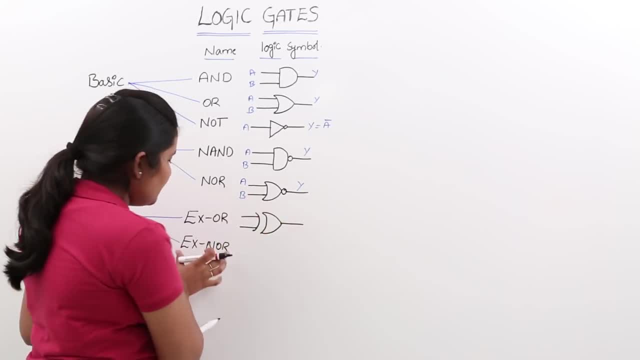 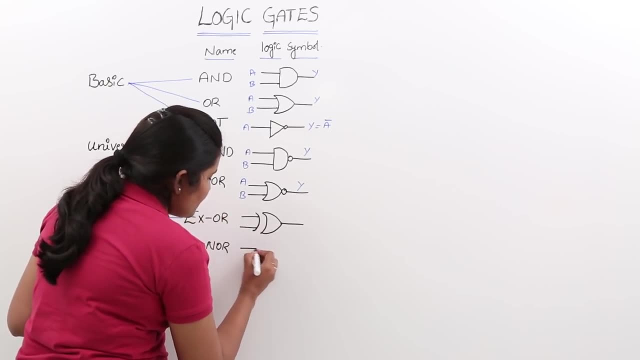 identify this as XOR gate. So here XNOT. we can say this: XNOT gate is complement gate for XOR gate. That means whatever here you are having as XOR gate for that if you take in any bubble here, not here, it will gives you symbol, logic symbol for XOR gate. 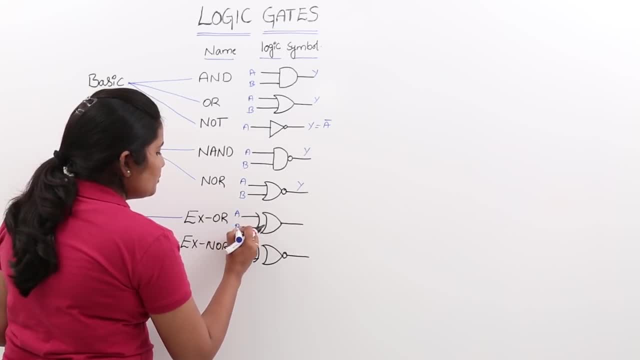 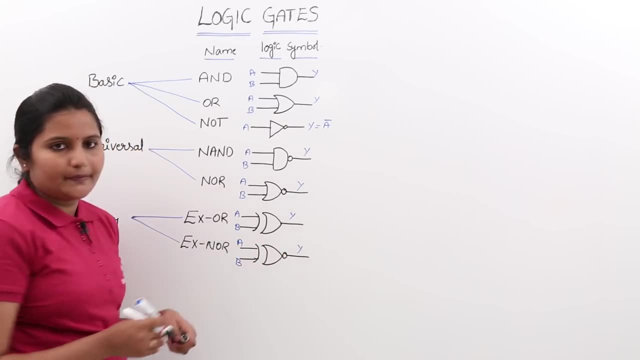 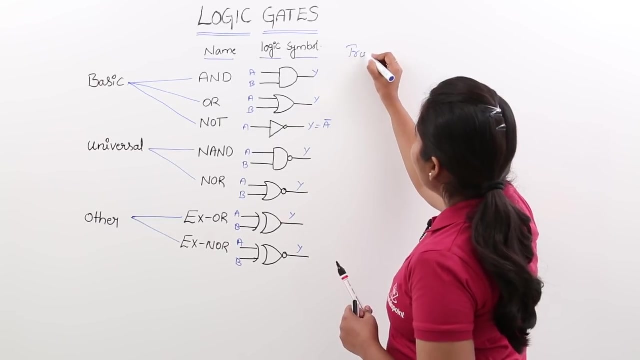 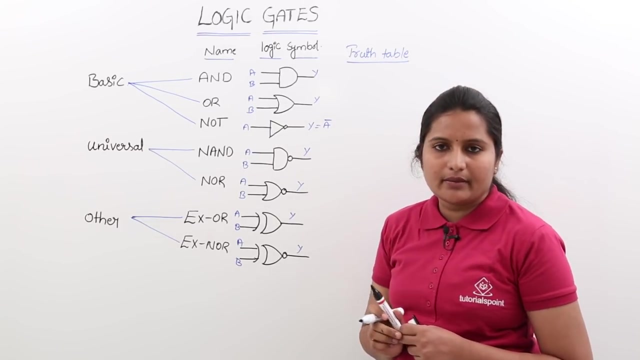 So here also we are having two inputs A and B, one output Y. Here also you are having two inputs A and B, one single output Y. Now we will skip in to truth tables. So here we know that truth table is going to provide the input output relation. Truth table will defines what may. 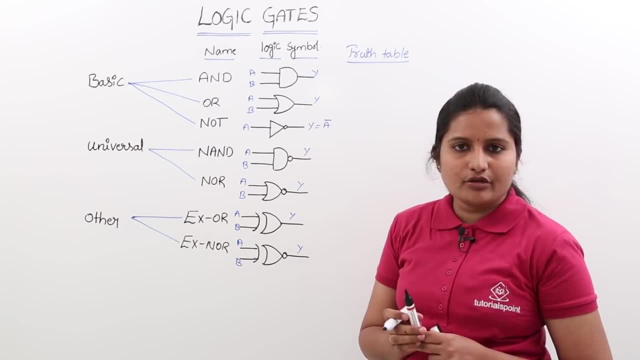 be the output of logic gate for particular gate. Why logic gate is given particular gate for specific gate. What logic gate is there and what magic gate for specific gate? ae, Here you are: combination of input, So truth table always contains columns, which is having inputs, and 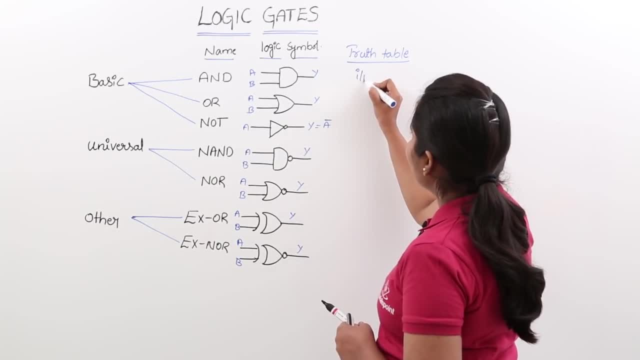 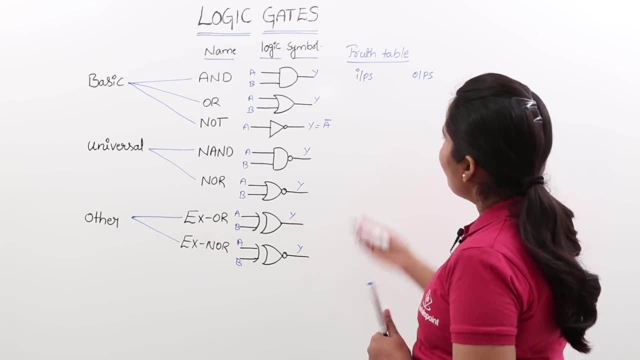 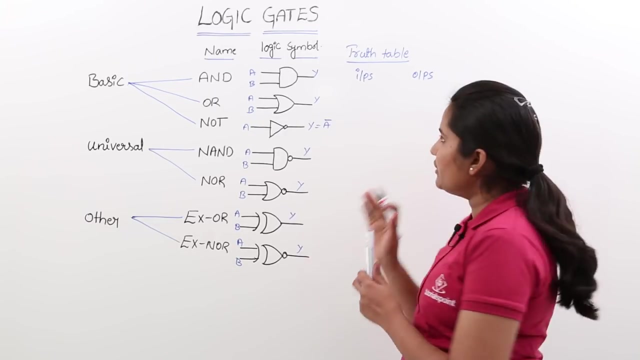 outputs. So here I am having inputs and I am having outputs in truth table. So here, in truth table, what are the inputs means? whatever we are having at input of gate, that all you need to take at input columns, For example, if you are taking for end gate or OR gate, what are the inputs means? 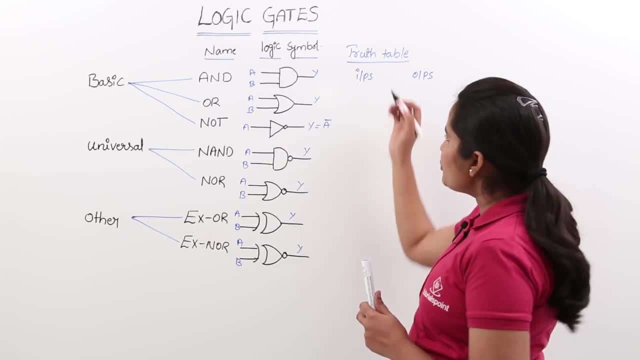 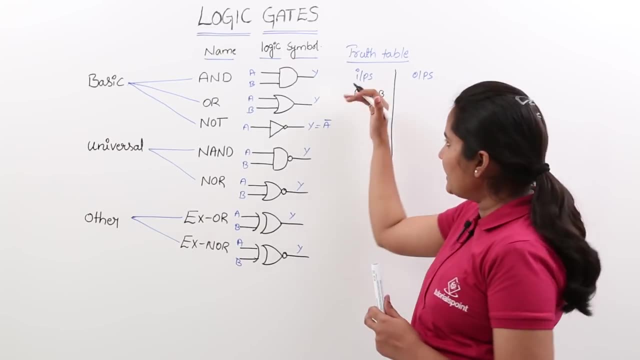 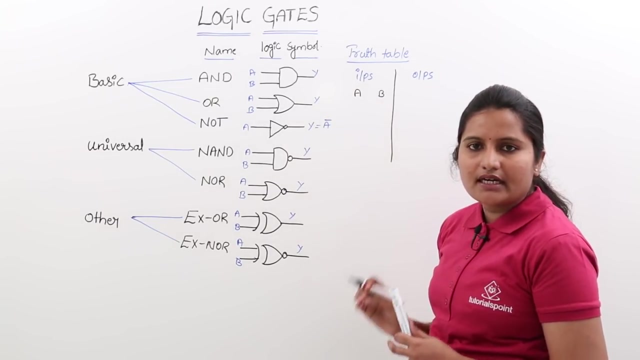 A, B are the inputs in each and every gate. So truth table includes A and B in inputs column. So we will take the combinations for that: inputs, So next in output. so whatever you represented at output that you are going to take as output. So by completing this truth, 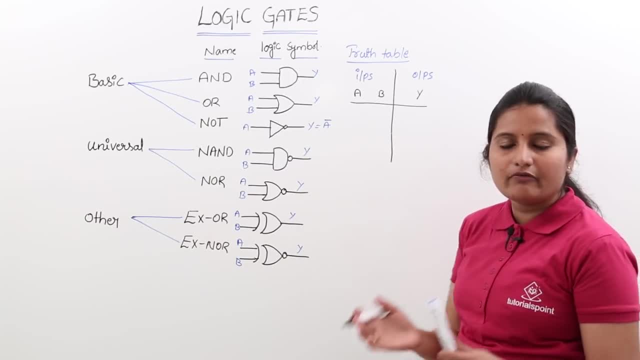 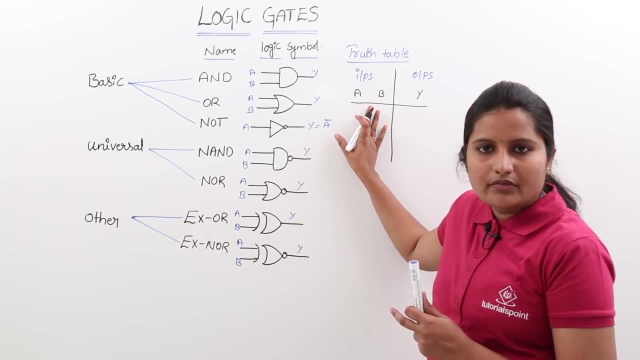 table you are going to take the combinations for that inputs, So next in output, so whatever, by seeing itself we can say what is the output for particular combination of inputs. So now, how many combinations we may have here? How many combinations means? So 2 power n. 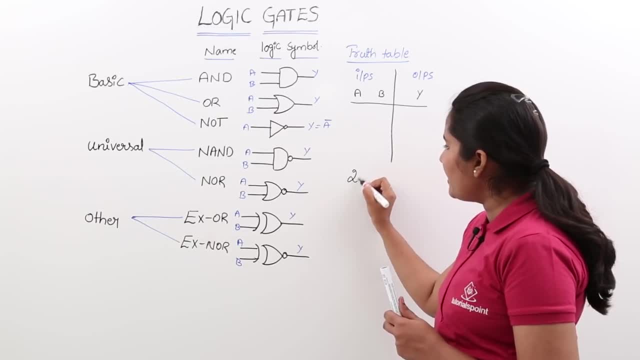 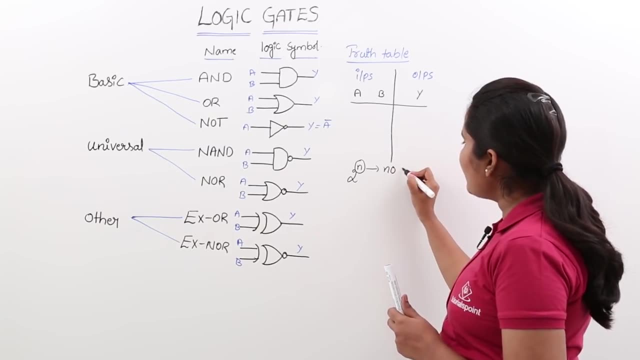 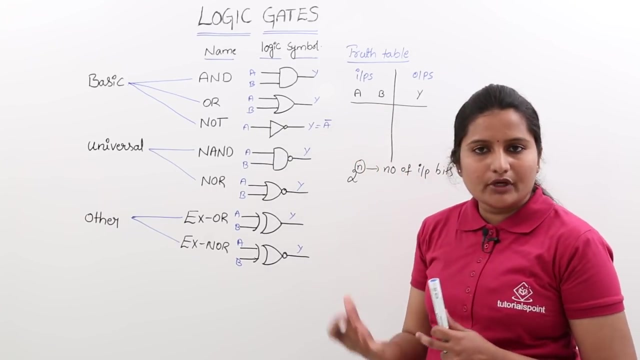 combinations we may have. So this 2 power n, in which this n is equivalent to number of input bits, So this is number of input bits. So now, for example, if you are taking, for example, if you are taking 2 input end gate, the number of inputs is 2.. So, as our number of inputs is 2, 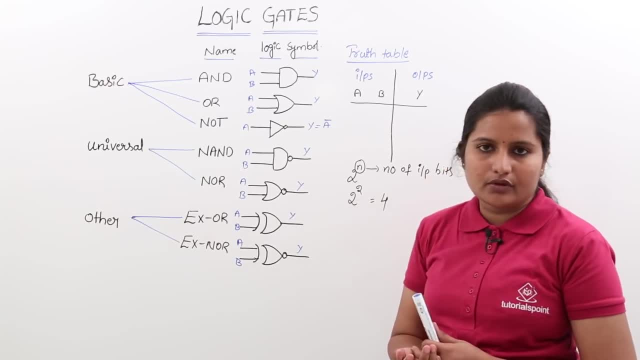 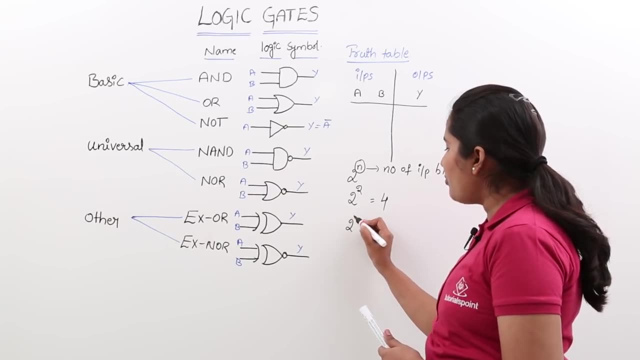 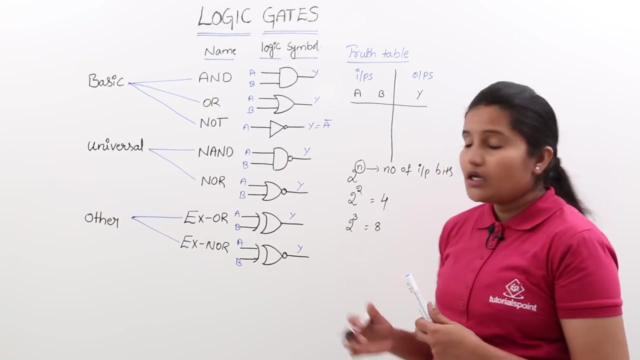 you may have 4 combinations of that input. For example, if you are having 3 input end gate or 3 input gate, you may have 2 cube combination of inputs. in truth table that means 8 input combinations. you may have. that means A, B, C. you will get 8 combinations Now. 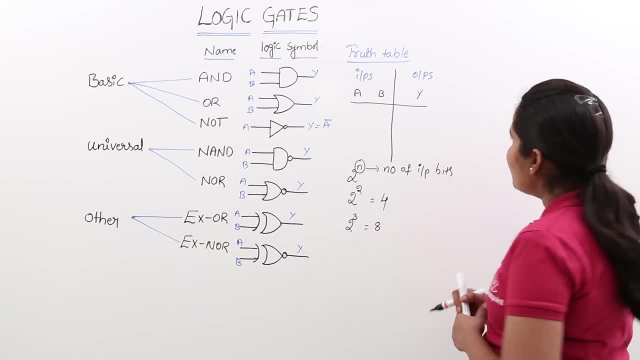 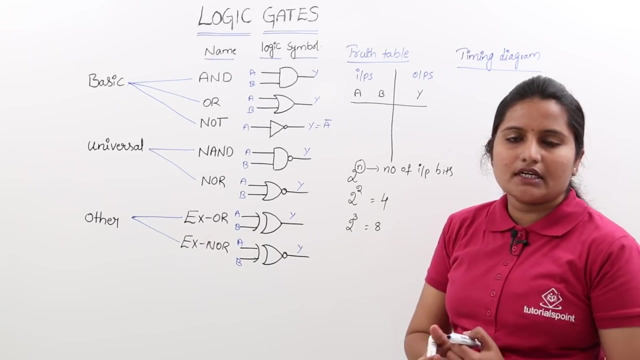 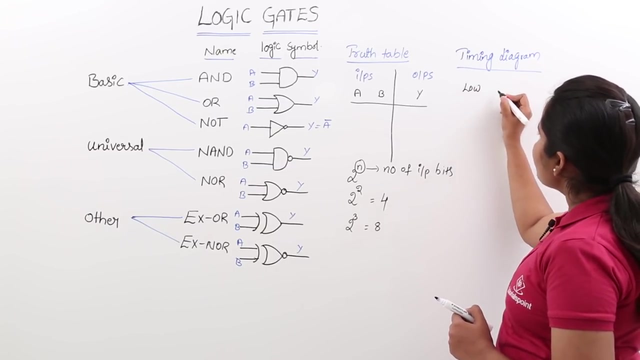 we will skip into timing diagram. So this timing diagram is also very, very important. Timing diagrams are nothing but diagrammatic representation of input and output. Diagrammatic representation of input and output. So here low level will be represented like this. So 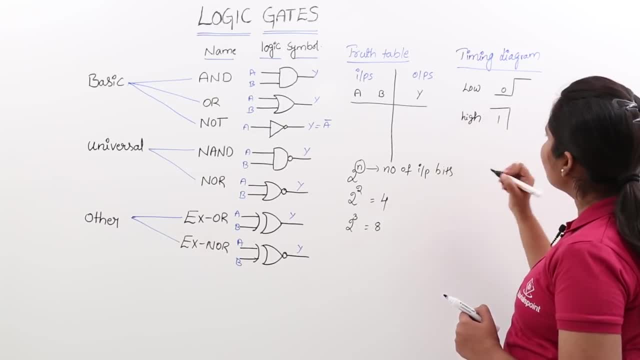 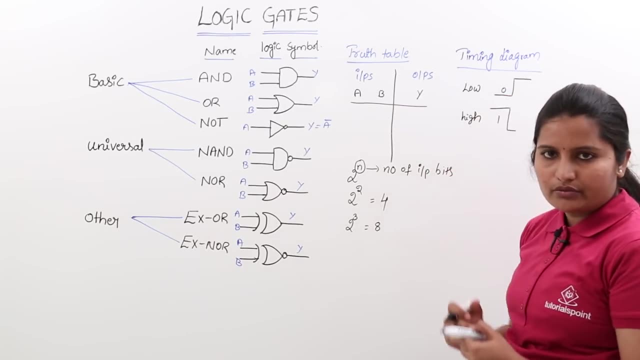 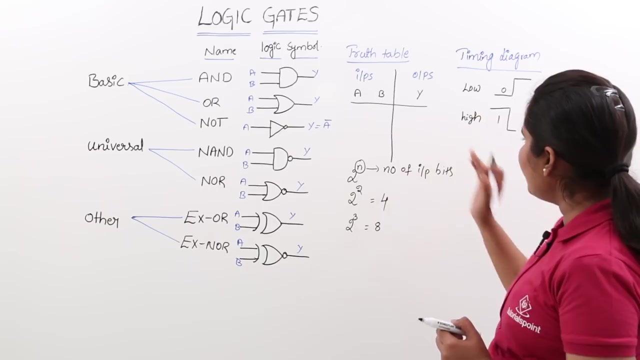 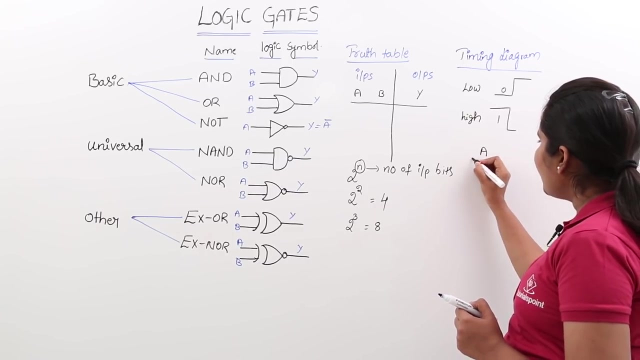 this is high level, So high level will be represented in high pitch and low level will be taken it down. So now, by using this, we are going to draw some timing diagrams. So here, for example, if you want to draw timing diagram for A, So A is 0, after that at a T1: 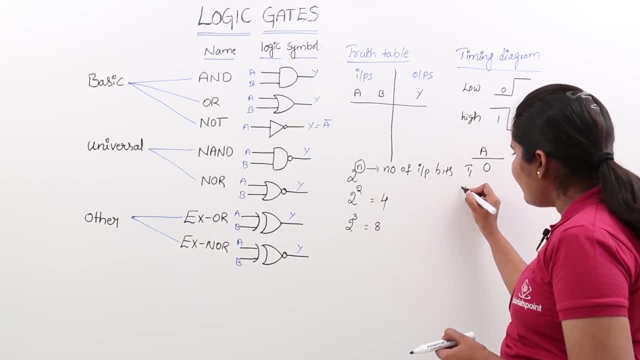 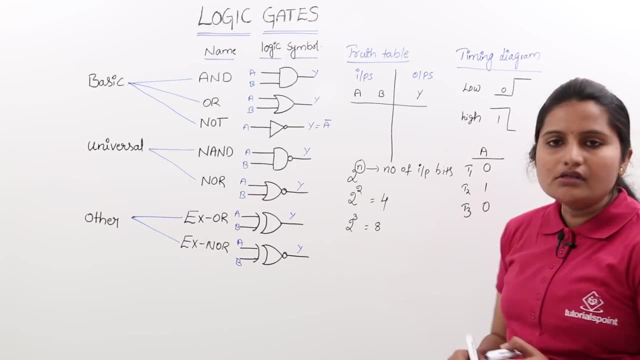 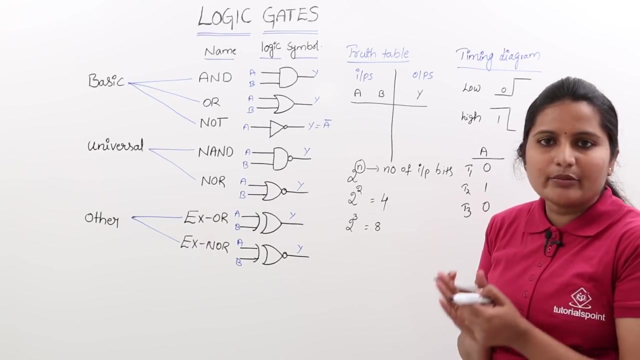 time cycle A is 0. And T2 time cycle A is equivalent to 1.. At T3 time cycle, again, it is pulled down to 0. For example, if you want to draw the diagrammatic representation of A, that means time cycle. 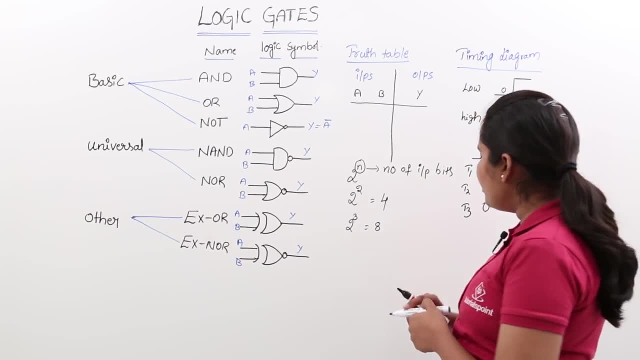 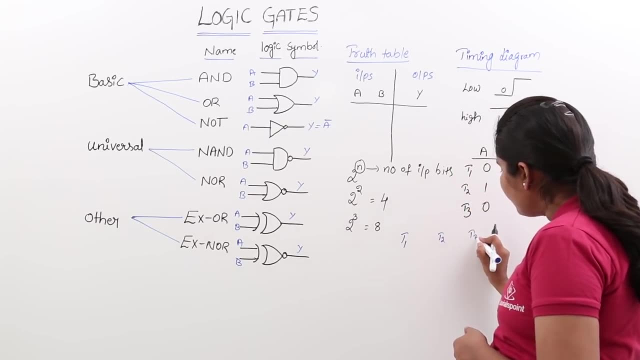 at each and every time period. first of all, you need to take that time period. that means T1 and T2 and T3.. So I am just taking the barriers like this. So T1 is up to here, T2 is up to here and 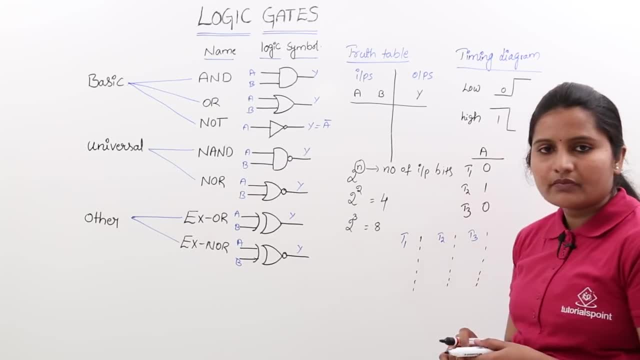 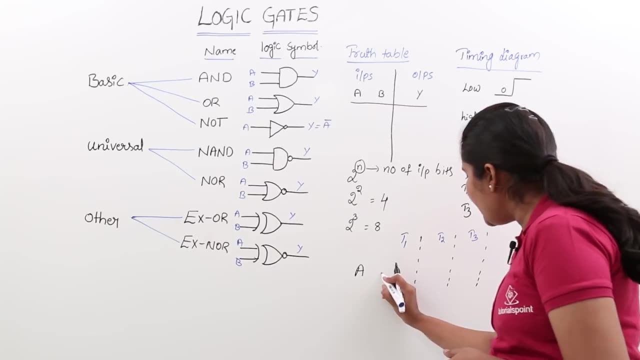 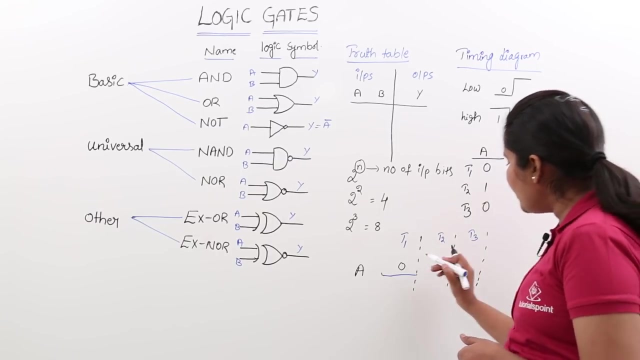 T3 is up to here. So now if you want to draw A, then A at T1 is equivalent to 0. I am just making this as 0. So this is 0. And A at T2 is pull up to 1. that means it rises to. 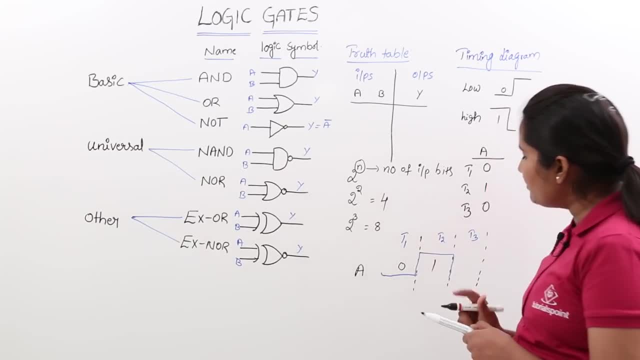 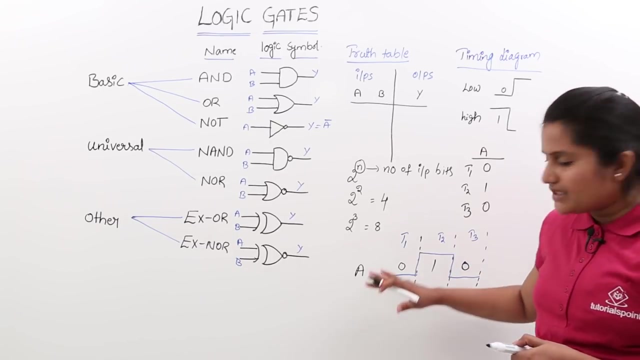 1. So this is 1 here. So now T3: at T3 this A value is equal to 0. that means again, this is down to 0.. The value here is equivalent to 0 here, So this is called as timing diagram. 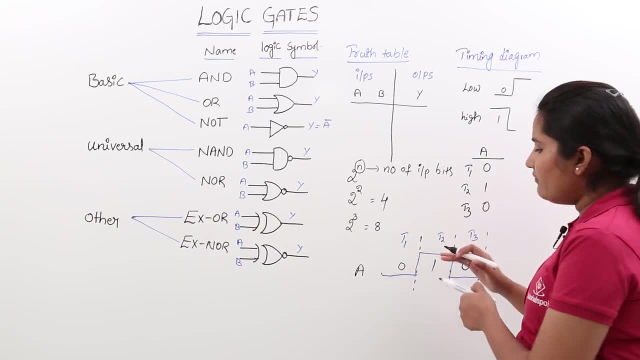 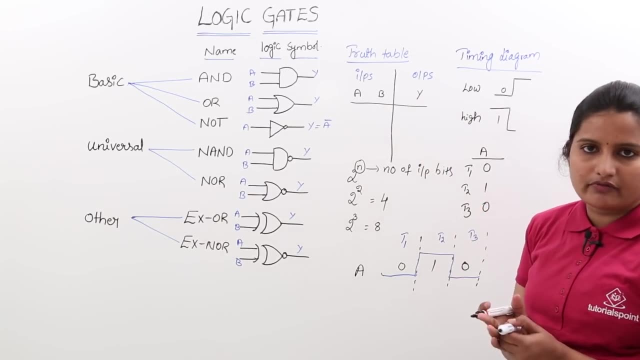 for a variable A. So in the same way we can have different timing diagrams for all truth table variables. that means input, output variables. So in exams we may get questions on truth tables and timing diagram also, sometimes one mark questions we may get like this, So they will simply give the functionality in truth. 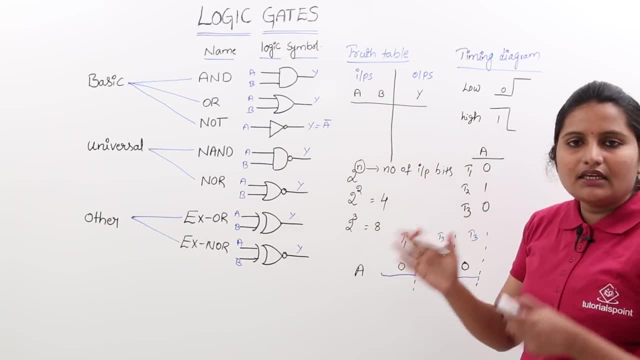 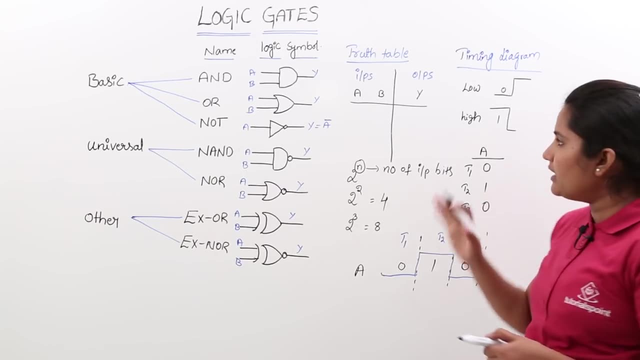 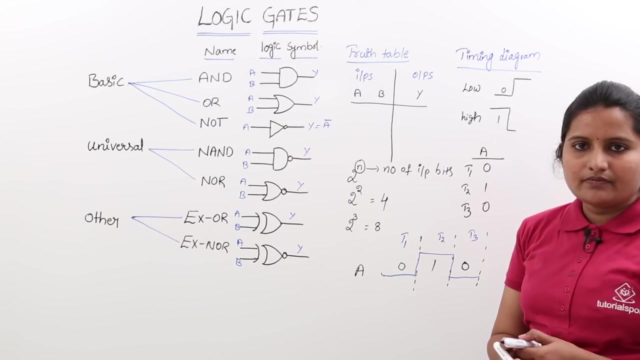 table. they will provide the values in truth table. by seeing the values itself, we have to say this is related to so and so gate. And similarly they will provide timing diagrams also. So by observing the timing diagrams, we have to say this is related to so and so gate. 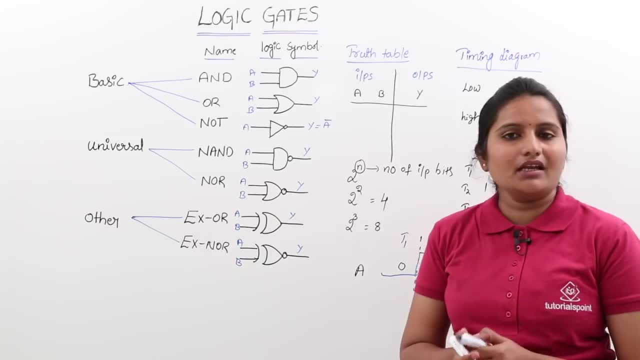 So like this, we are getting questions on this basic logic gates.